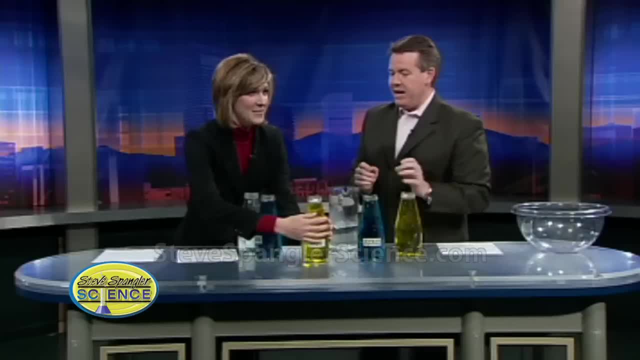 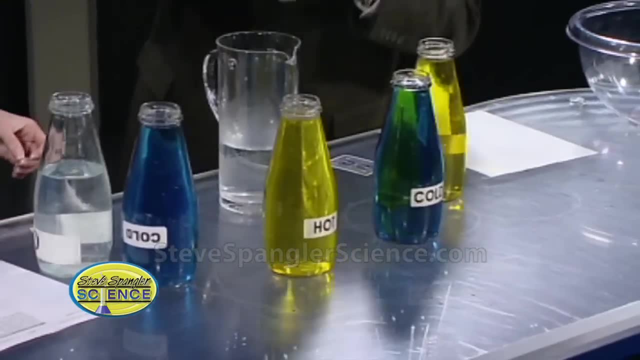 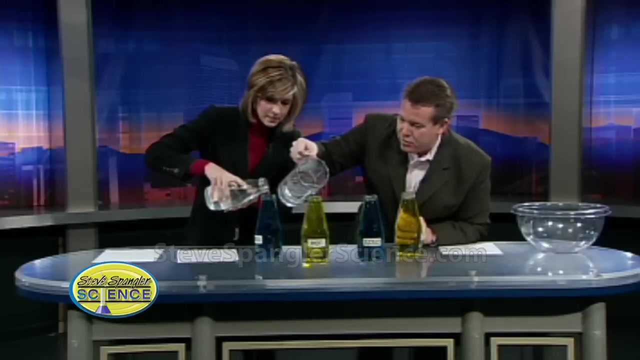 Yeah, I was like colder than it was outside. So here's the warm water right here. So let's set up some scenarios. One of the scenarios is the warms on the bottom, So the sun heats the earth and that hot air kind of rises, And so let's do this. If you'll take the cold and fill this up, I'm going to take the warm and fill this up And then somehow we've got to maneuver that cold over the top. All right, so put the 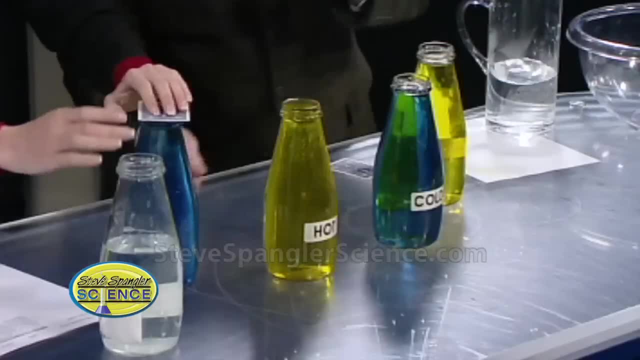 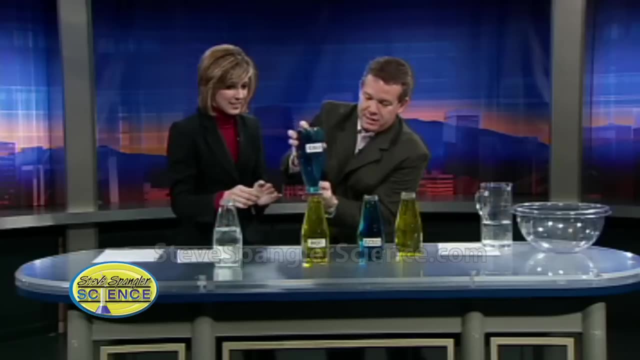 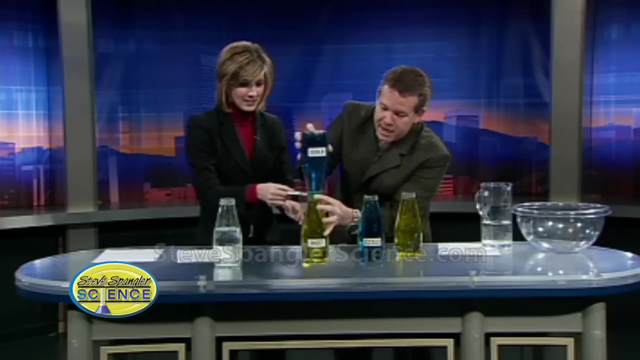 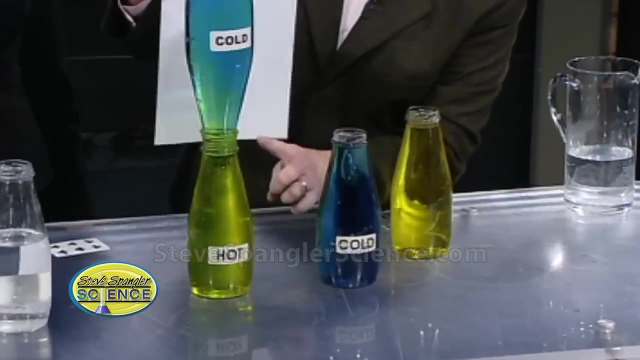 rain card on top of the cold. Feeling good about this, No, Wearing your best clothes? Yes, of course. Okay, I'm going to help you with this. I'll turn it upside down and then you're going to pull the card out of the way. Okay, so ready. So card goes upside down like this: Yeah, All right. And so right on top, like this: And now you slowly just pull the card away. Go ahead Slowly, Yep, just kind of pull it away. Nice, Good. And now we get this beautiful color mixing Right. You see the mixing that's there. The warm goes up, just like the air would, and the cold goes down. And so they say: this is a pretty good reason for. 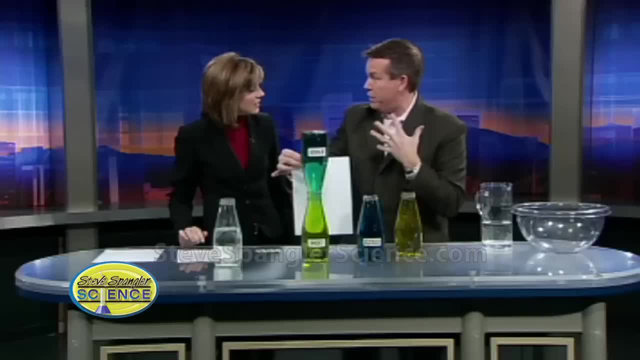 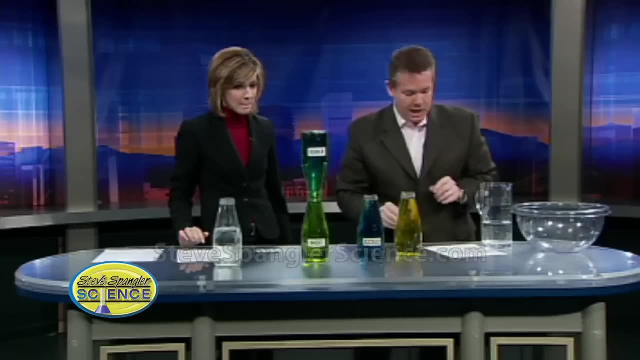 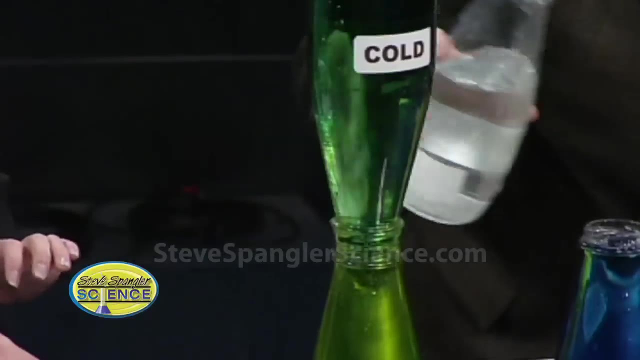 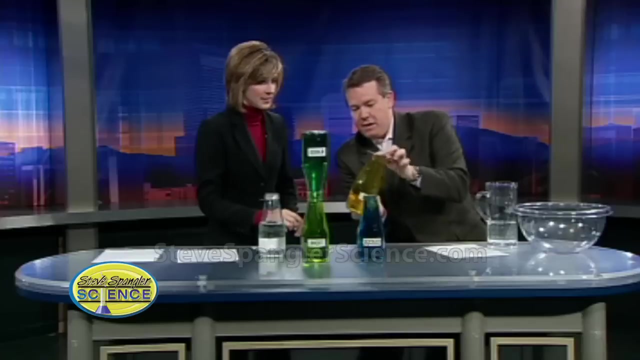 daylight savings in terms of us driving. You want to drive when there's light out, Right, Because you want the earth kind of warming and you want the gases moving back and forth- Exactly, Be very careful not to sneeze. We're going to go for this one, All right. So here we go. Here's the warm. now It's going to sit on the top Right, And the cold will sit on the bottom, And this is where we start to get that temperature inversion. Okay, All right. So here we go. So this guy sits on top here like this. Okay, Upside down. All right, Stay there, Stay there. All right, Here we go. And now we pull out of the way And watch what happens. We 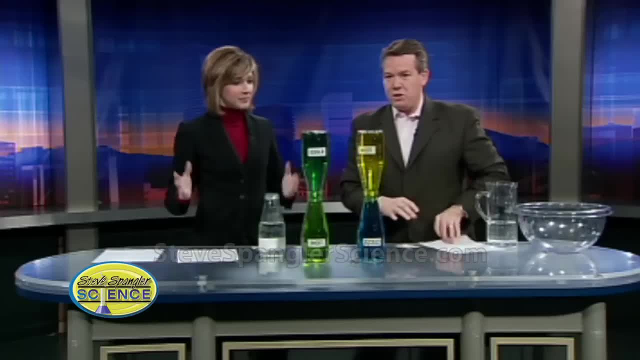 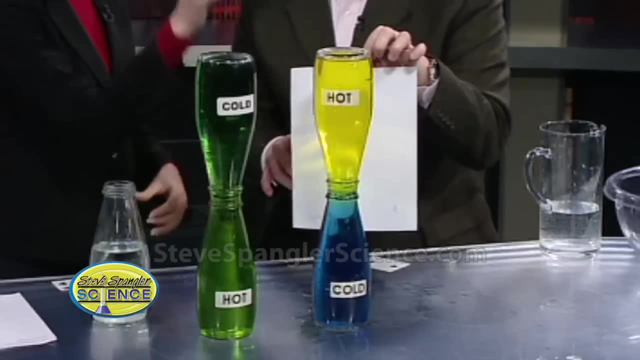 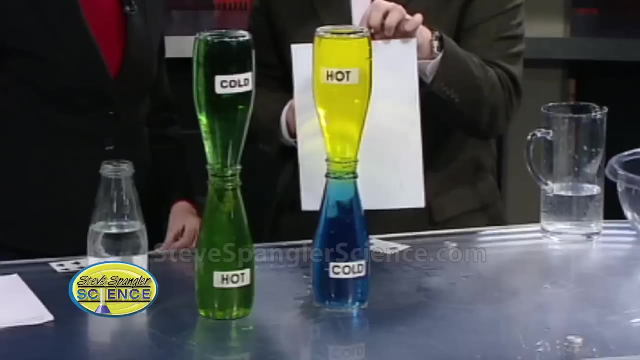 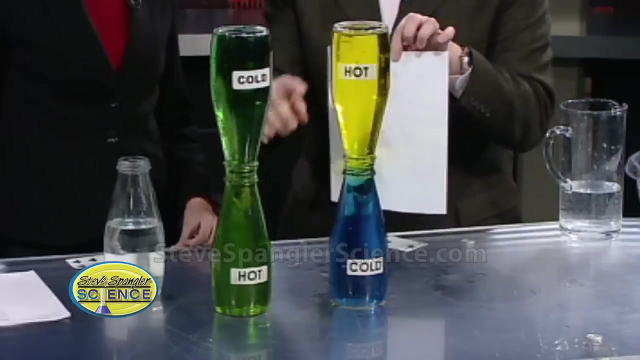 get next to no color mixing at all. So you kind of see what the difference is there. Isn't that kind of fun. So when we have that inversion, all of that ick kind of stays in the cold air Exactly right With the warm air, So that warm air literally traps it down below, And so no wonder the pollution is bad. You see that layer that's right there in the middle, Yep. So what a great way to be able to see that concept of temperature inversion. Teachers also talk about convection that we're seeing here. We want the convection in the atmosphere. We don't want this temperature inversion that you kind of see here. But I think it's just a startling demonstration with. 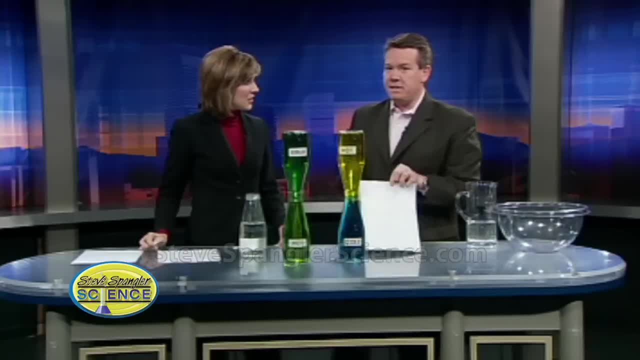 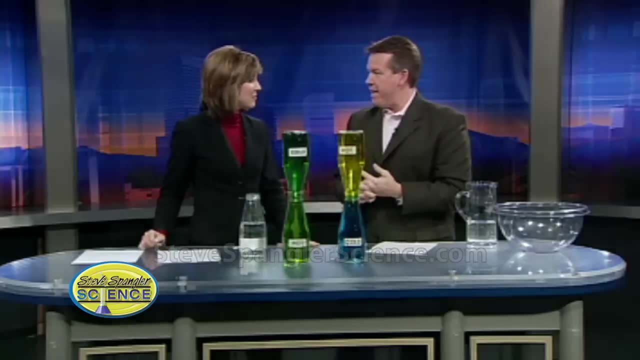 the green that sits over here like this, I know, And then as it sits over, this way it's kind of a cool way to be able to see it And it's simple, little bottles- Great way to see exactly why some days it just looks kind of nasty over Denver and why some days it doesn't- Absolutely right.